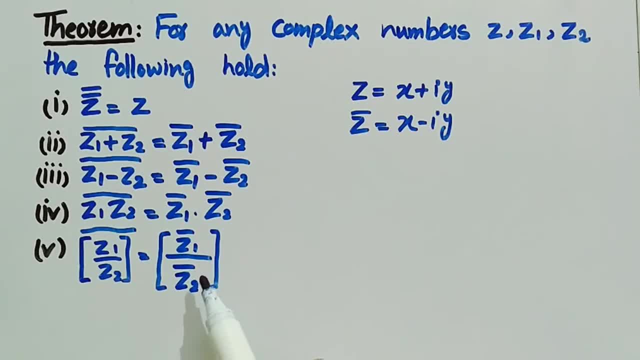 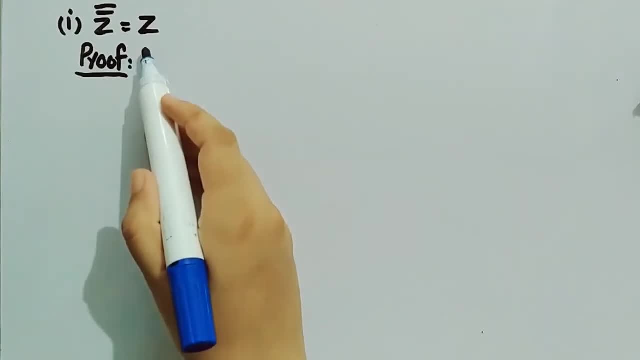 Now we will prove these properties one by one. The first one is: z double conjugate is equal to z. To prove it, we let z is equal to x plus iota y. Then z conjugate is equal to x minus iota y. Z double conjugate will be equal to x minus. iota y minus y, which will be equal to x plus iota y. Then z double conjugate will be equal to x minus iota y minus y, which will be equal to x plus iota y, Which is equal to z. So z double conjugate is equal to z. 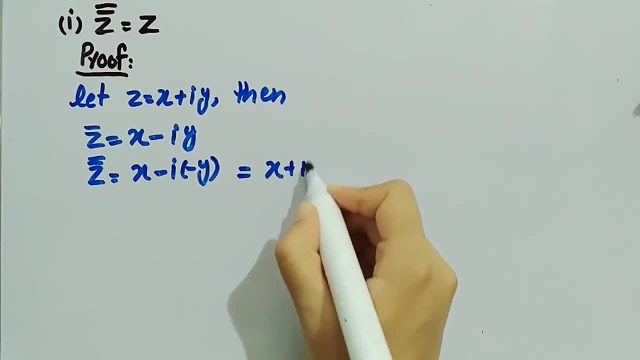 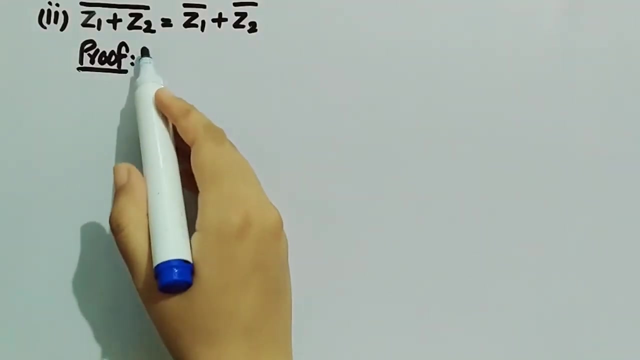 The second property is z1 plus z2. whole conjugate is equal to z1 conjugate plus z2 conjugate. For this let's consider: z1 is equal to whole conjugate is equal to z1 conjugate plus z2 conjugate. 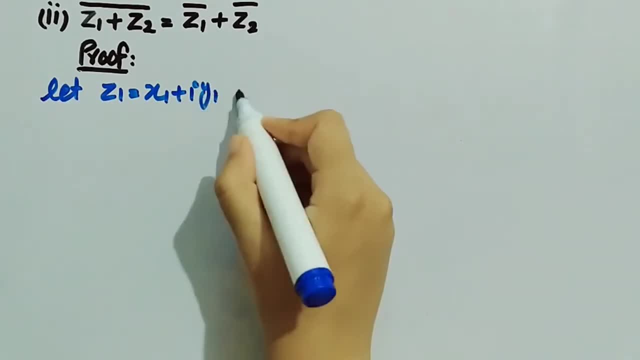 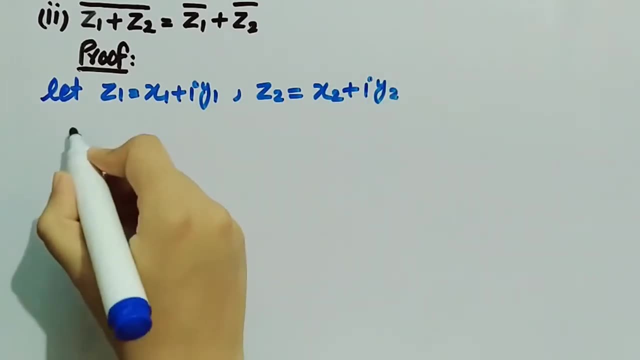 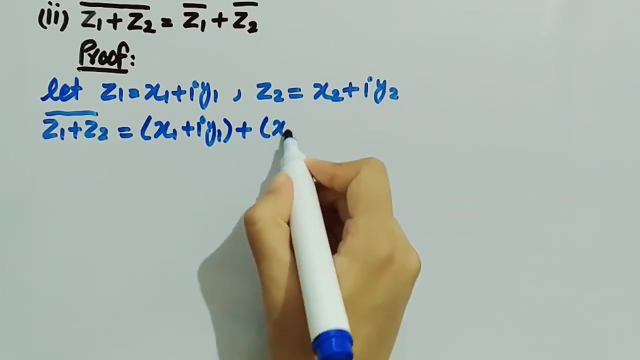 x1 plus iota, y1 and z2 is equal to x2 plus iota y2. now for z1 plus z2 whole conjugate, we will write values of z1 and z2 which are x1 plus iota, y1 plus x2 plus iota y2 whole conjugate. 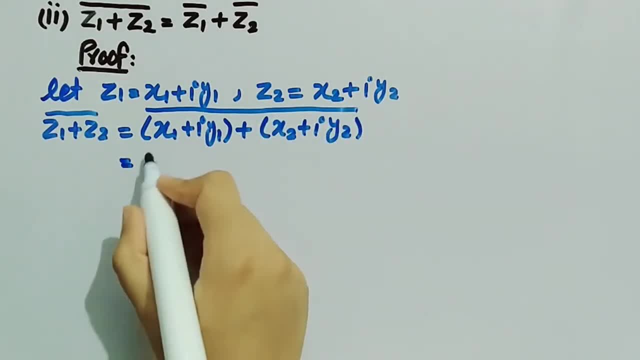 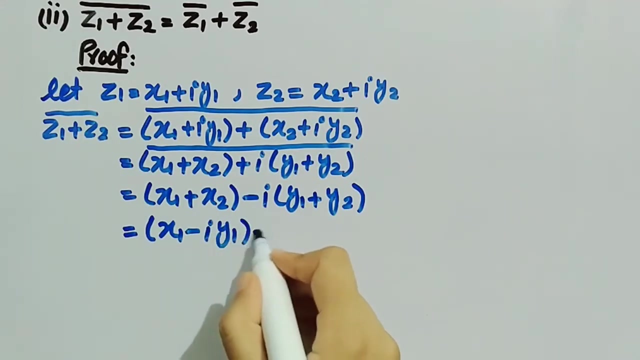 now we will rearrange them and get x1 plus x2 plus iota y1 plus y2 whole conjugate. now we will apply conjugate and get x1 plus x2 minus iota, y1 plus y2. now we will rearrange it again and get x1 minus iota y1 plus x2 minus iota y2. 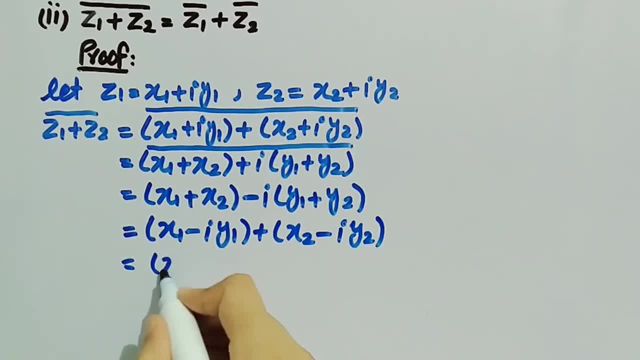 which is equal to x1 plus iota y1 conjugate plus x2 plus iota y2 conjugate, which is equal to z1 conjugate plus z2 conjugate. so this property is proved. now we will prove the third property, which is z1 minus z2 whole conjugate is equal to: 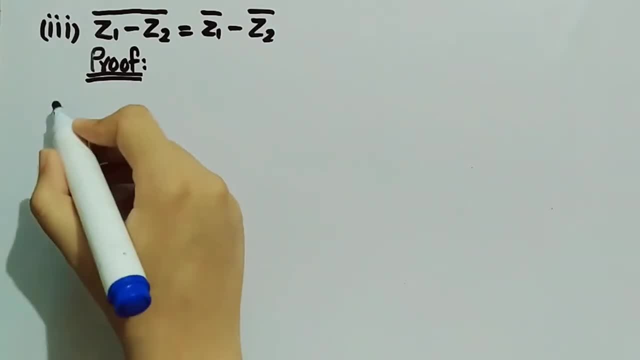 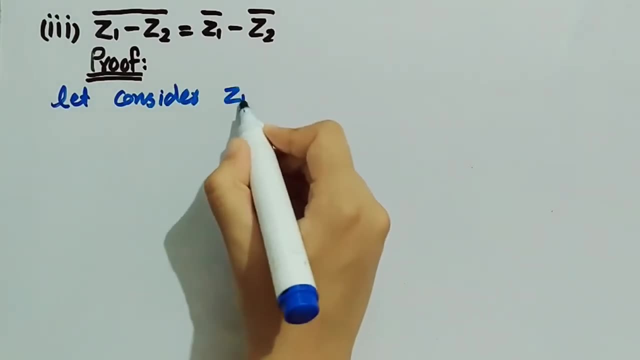 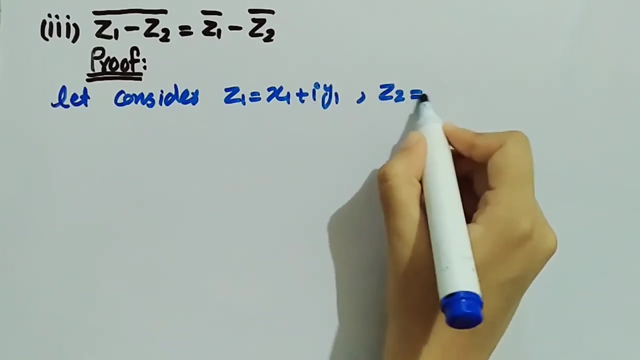 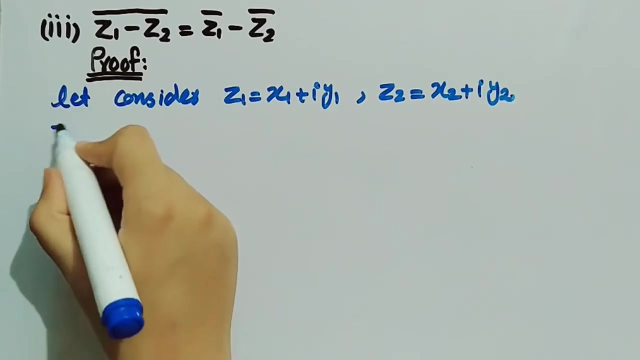 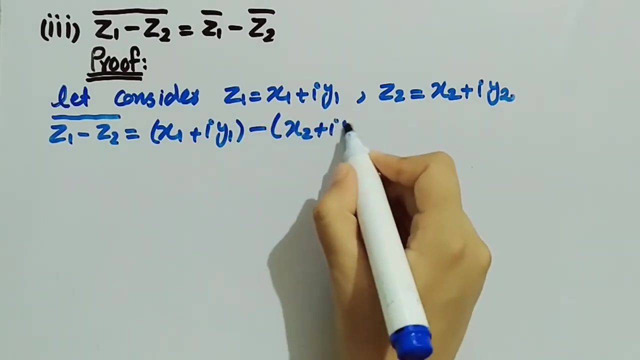 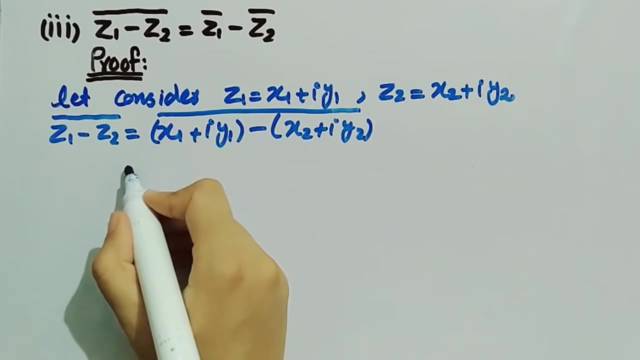 z1 conjugate minus z2 conjugate. for this, let's consider: z1 is equal to x1, iota y1 and z2 is equal to x2 plus iota y2.. z1 minus z2 whole conjugate will be equal to x1 plus iota y1 minus x2 plus iota y2 whole conjugate, which will be equal to, after rearranging: 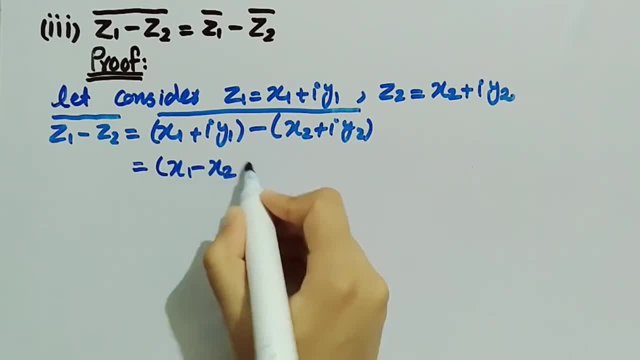 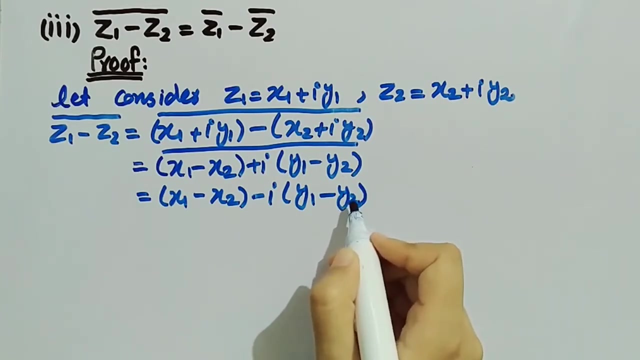 x1 minus x2 plus iota y1 minus y2, whole conjugate. After applying the conjugate, we get x1 minus x2 minus iota y1 minus y2, now we will rearrange it and we get x1 minus iota y1 plus minus x2 plus iota y2.. 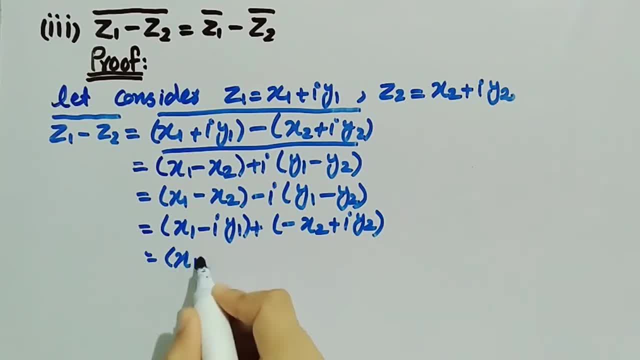 Which is equal to x1 minus iota y1.. Now, taking the minus sign common, we get x2 minus iota y2, which is equal to x1 plus iota y1 conjugate, minus x2 plus iota y2 conjugate, Which is equal to z1 conjugate minus z2 conjugate. 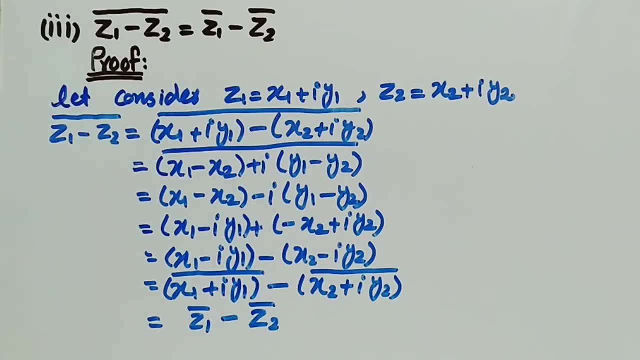 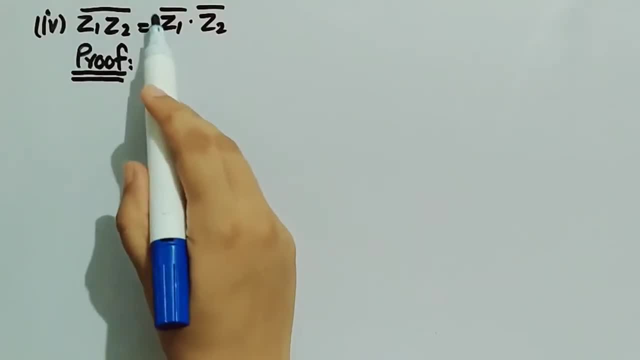 So this is the proof of third property. The fourth property is: z1 multiplied by z2 whole conjugate is equal to z1 conjugate multiplied by z2 conjugate. For this let's consider: z1 is equal to x1 plus iota y1.. 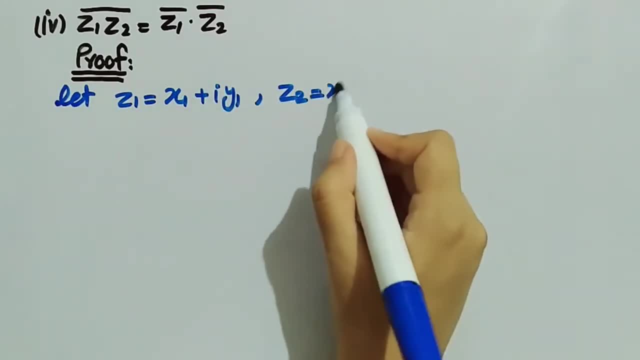 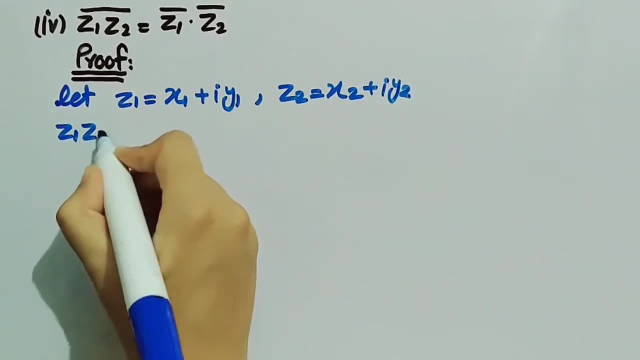 z2 is equal to x2.. x2 is equal to x1 plus iota y2.. Then z1 multiplied by z2 whole conjugate will be equal to x1 plus iota y1 multiplied by x2 plus iota y2 whole conjugate. 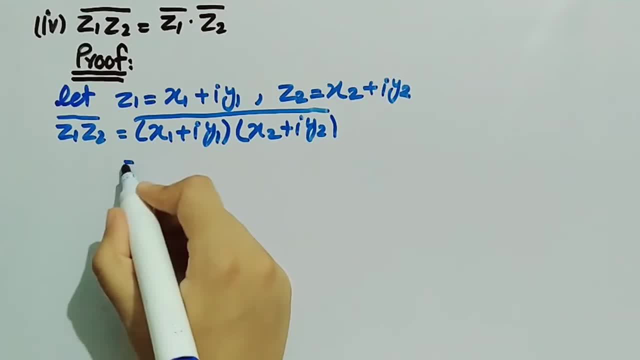 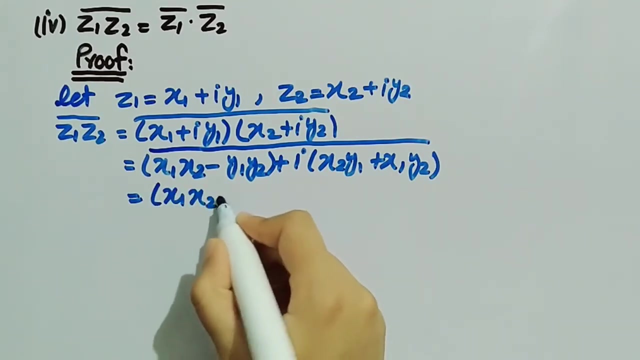 minus y1- y2 plus iota, x2- y1 plus x1- y2.. This is the value that we got after multiplying these two complex numbers and whole conjugate. After applying conjugate, we get x1- x2 minus y1- y2. 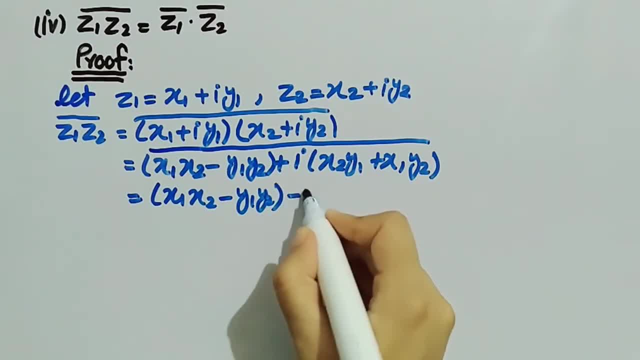 minus iota x2, y1 plus x1 y2, which is equal to x1 minus y1 y2.. We can also write it as x1 plus iota y1 conjugate multiplied by x2 plus iota y2 conjugate, which is equal to z1 conjugate multiplied by z2 conjugate. This is the proof of fourth property. 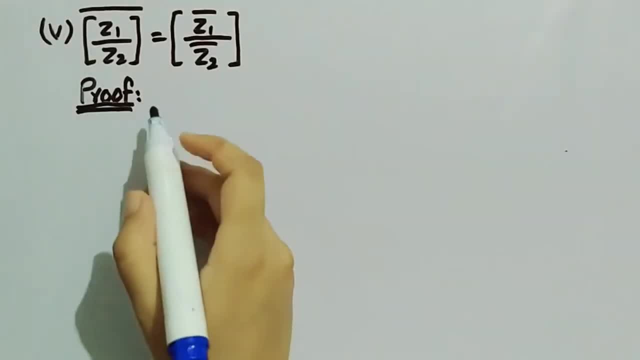 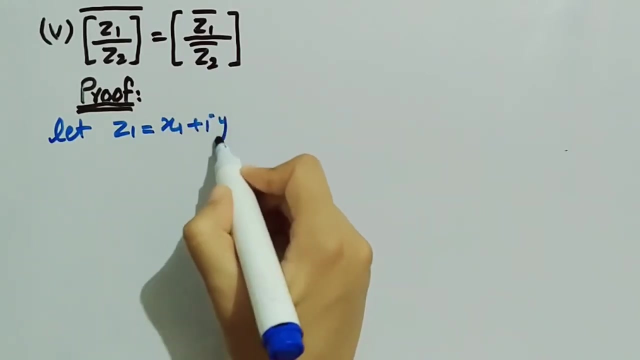 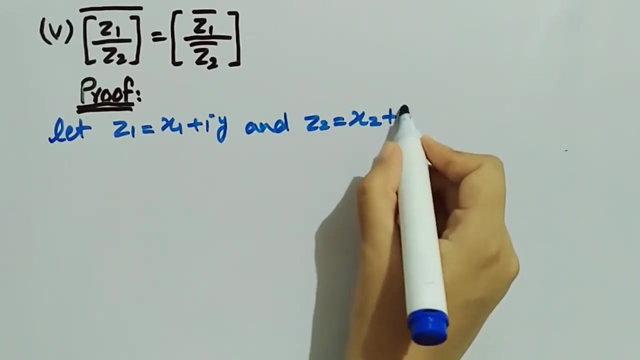 The fifth property is z1 divided by z2. whole conjugate is equal to z1 conjugate divided by z2 conjugate. Firstly, let's consider: z1 is equal to x1 plus iota y1 and z2 is equal to x2 plus iota y2.. 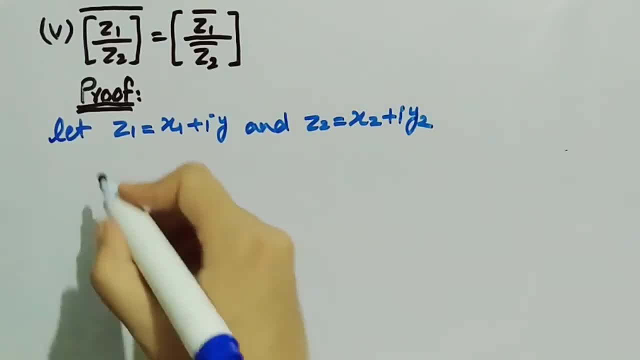 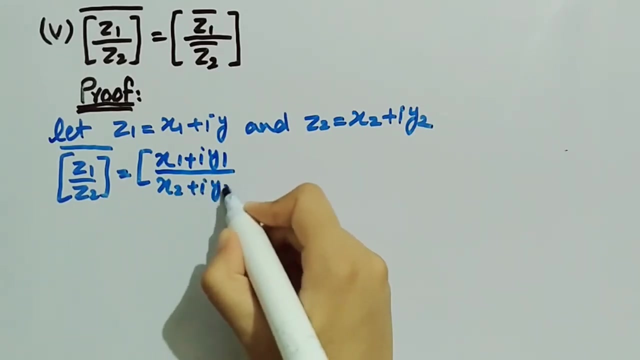 Now take z1 divided by z2 whole conjugate and it will be equal to x1 plus iota y1 divided by x2 plus iota y2 whole conjugate. Now x1 plus iota y1 divided by z2 whole conjugate is equal to z1 plus iota y1 and z2 is equal. 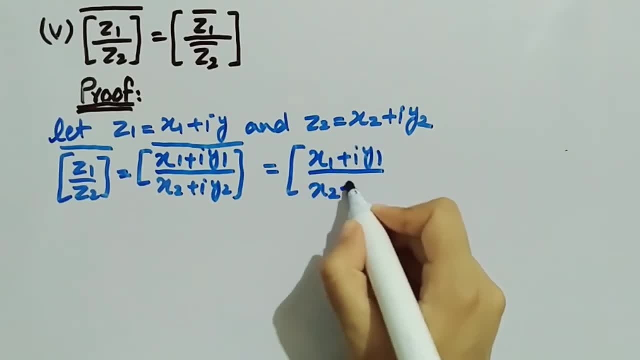 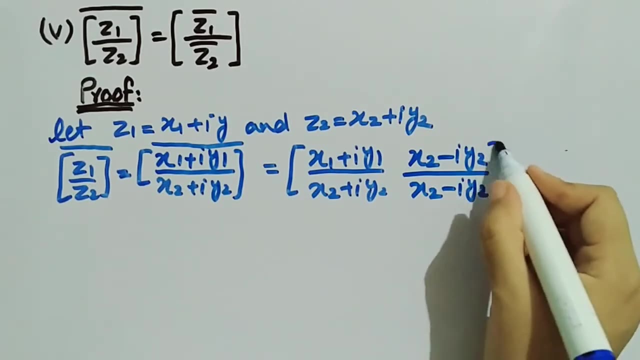 to z1 plus iota, y2, whole conjugate. Now multiply and divide it by x2 minus thì y2. now multiply and divide it by x2 minus diffusion r y to, x2 minus yota y to, and take whole conjugate: it is equal to. 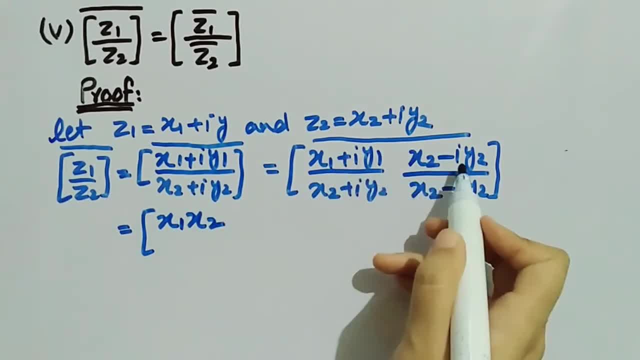 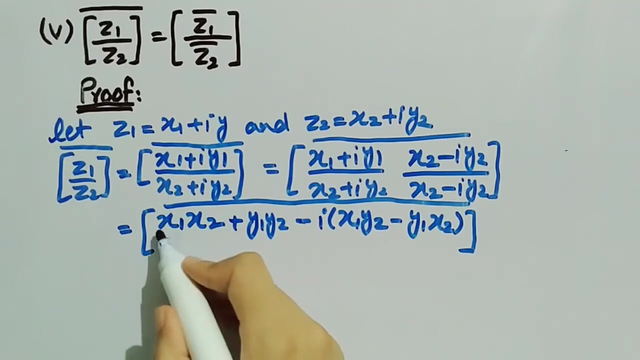 x1- x. Now we will x2. terms and write the answer here: y1 y2 minus iota, x1. y2 minus y1- x2. in previous video i have told you that how we can multiply any two complex numbers. so if you do not know how to multiply to complex number, then you can check out previous videos. 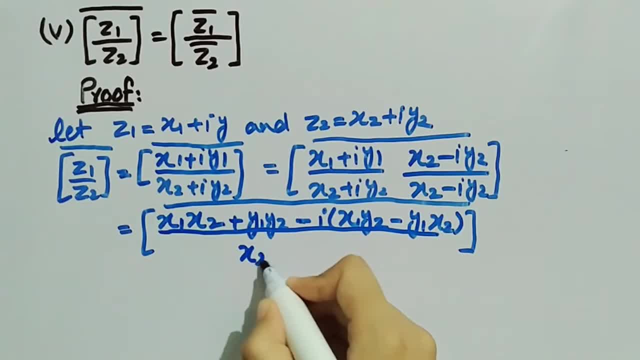 divided by x 2 square minus y 2 square, and it is equal to x 1 x 2 plus y 1 y 2, after applying conjugate minus iota will be changed to plus iota: x1y2 minus y1x2 divided by x2 square plus y2 square. Let's name this: 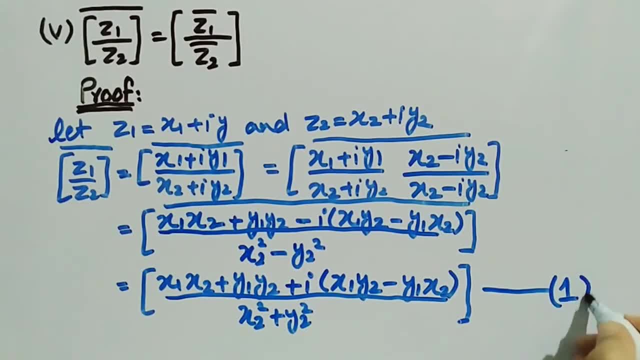 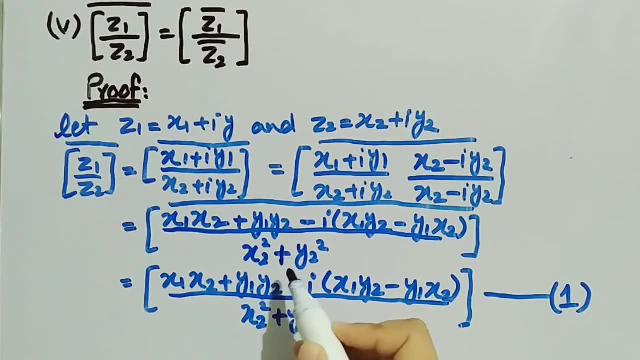 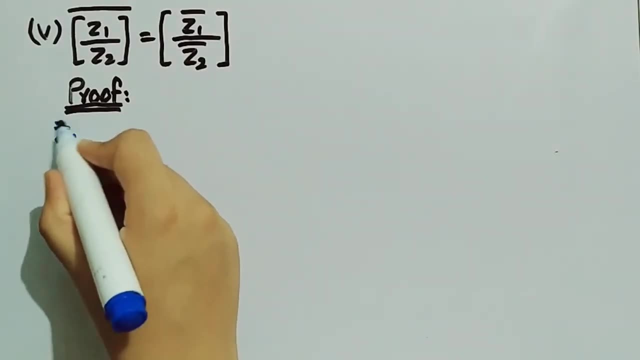 equation as equation 1.. Sorry, there is a mistake. this is also positive sign. Now take the other side, which is z1 conjugate divided by z2 conjugate, and it is equal to x1 minus iota y1 divided by x2. 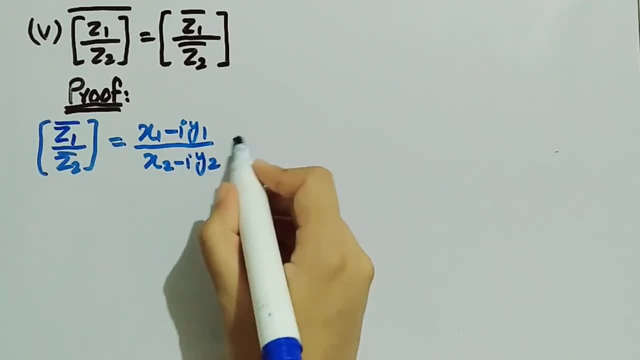 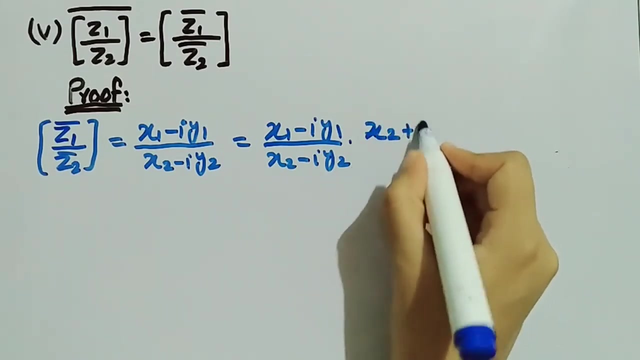 minus iota y2.. We will multiply it and divide it by x2 minus x2 plus iota y2 and we get x1 minus iota y1 divided by x2 minus iota y2.. x2 plus iota y2 divided by x2 plus iota y2.. 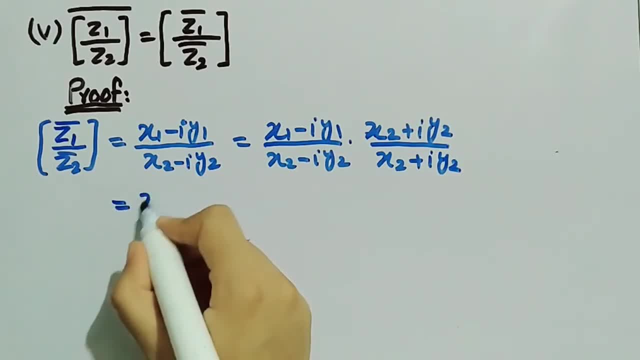 Which is equal to x1x2 plus y1y2 plus iota, minus x2y1 plus x1y2.. x1x2, y1x1x2, x1y2.. x2 1 and x2 1.. y2, 1, 2 pseudo where 1 is going over 1 plus 1 is going over 1 plus 1, 2 was equals to x1x2 plus yr2 plus iota y2, which is equal to x1x2 plus y1y2 plus iota x2. y1 minus x2y1 plus x1y2 divided by: 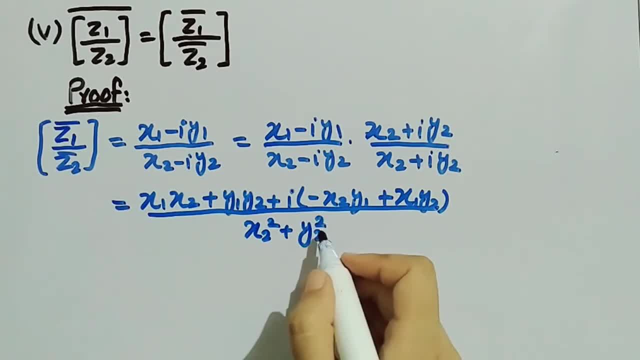 x1x2, Y1 plus x2y2 divided by x2 square: y1x2 plus x1Y2. square which is equal to x1, x2 plus y1, y2 minus iota, x1, y2 minus x2, y1 divided. 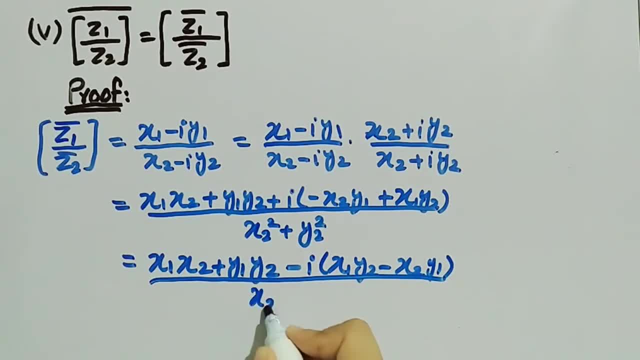 by x2 square plus y2 square. Let's name this equation as equation 2.. So from 1 and 2, we have z1 divided by z2 whole conjugate. z1 conjugate is equal to z1 conjugate divided by z2 conjugate. Hence proved: